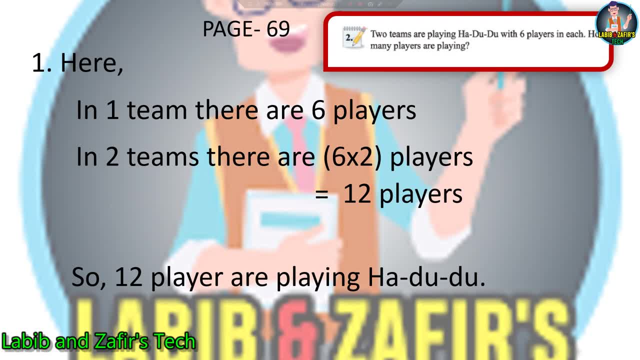 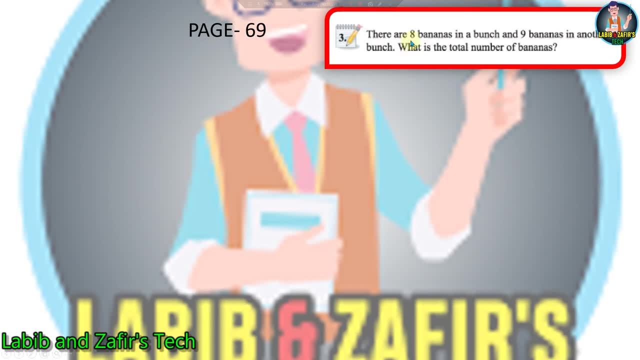 So, students, let's go to our next question. Student. this is again from page 69, and this is our second word problem. There are eight bananas in a bunch and nine bananas in another bunch. What is the total number of bananas? So, students, we can see that this is an addition word problem, So let's go through the word problem. 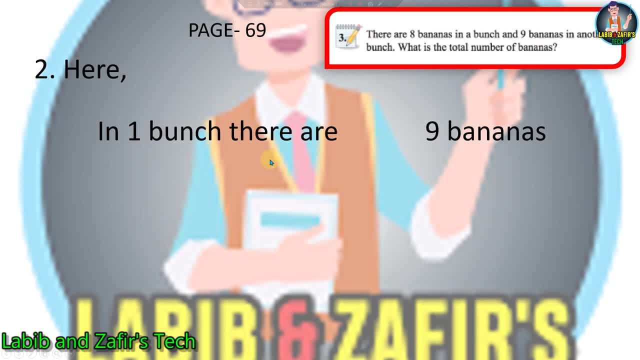 Number two here: In one bunch there are nine bananas, In another bunch there are eight bananas. So we can see in one bunch there are nine and in another there are eight. So we have to add this number. so total 9 plus 8 is equal to 17, because after 9, 10, 11, 12, 13, 14, 15, 16, 17, 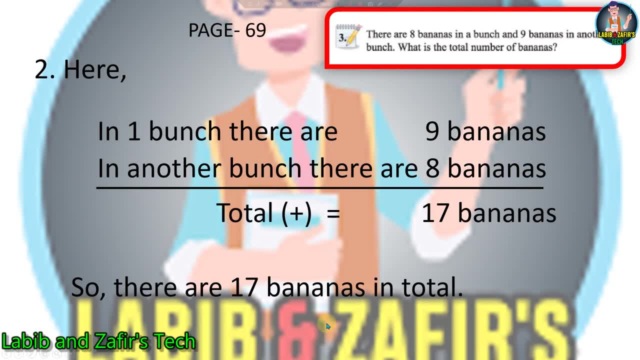 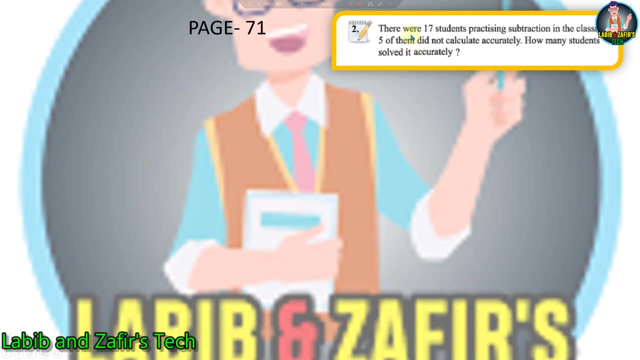 so that is, there are 17 bananas in total. so, student, this is our second word problem. now let's go to our third word problem, student. this is from page 71, so let's go through the question. there were 17 students practicing subtraction in the classroom. five of them. 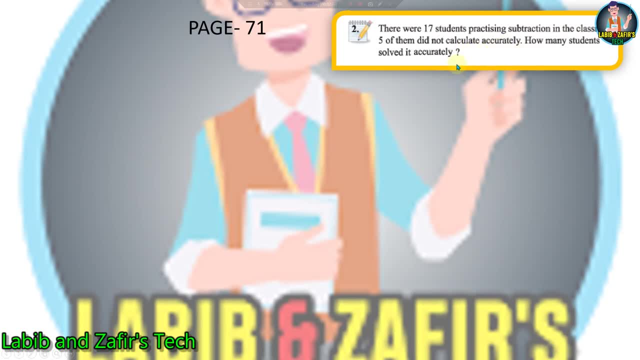 did not calculate accurately how many students solved it accurately. the students. we can see five of them did not calculate accurately how many students solved it accurately- the students. we have to find the number of students who have calculate the solve the math accurately or correctly. so let's go through the answer. 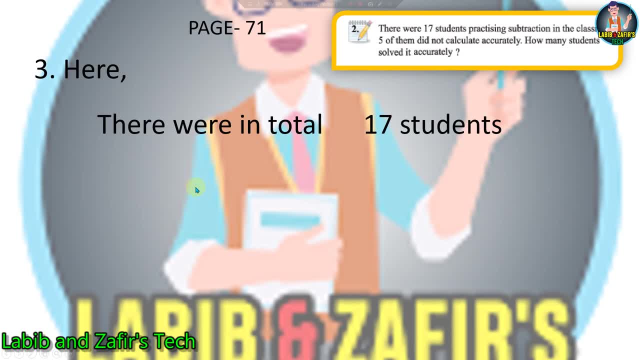 so number three: here there were in total 17 students. did not calculate accurately five students, so we have to do subtraction here. so if we do subtraction, that is if we subtract 5 from 17, that is 12, because if we add 12 plus 5 is equal that is 17, so left 12 students. 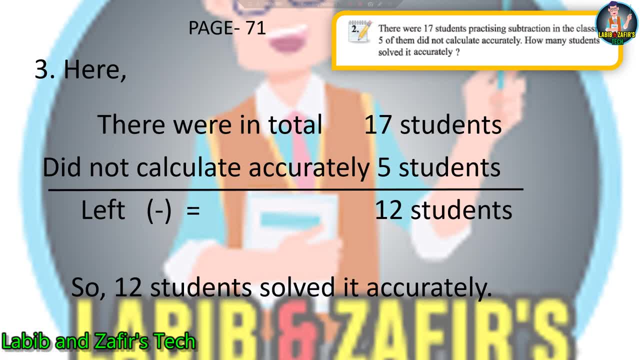 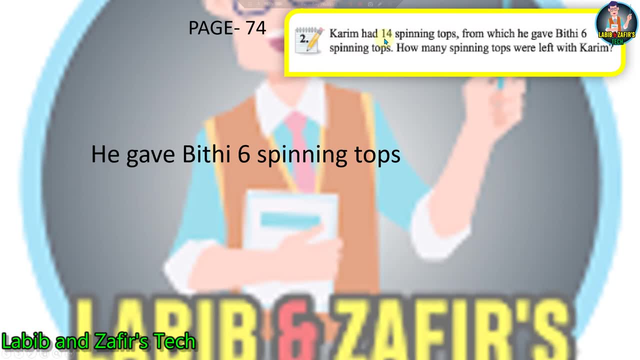 did not calculate accurately. so students list go to our fourth word problem. so students stated a mistake here. Corriegrave had 14 spinning tops, from which he gave be the six spinning tops. how many spinning tops were left with him, students? we can see here that Corrim had fourteen. 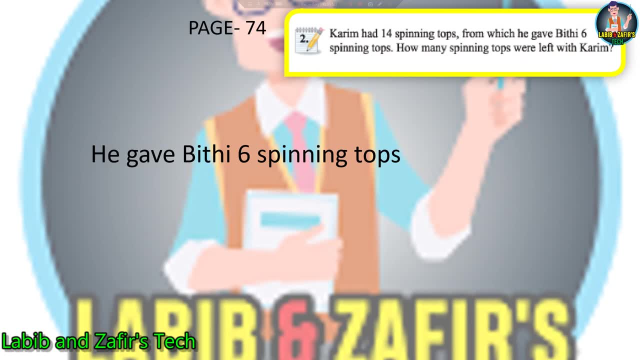 spinning tops and he, he gave beaten, Which are the dirty, 12 sabastians, so we have 12 Towerascals. Pity the number of spinning tops, so we have to find the number of drops remaining with Khorin. So here, number 4, Khorin had 14 spinning tops and he gave. 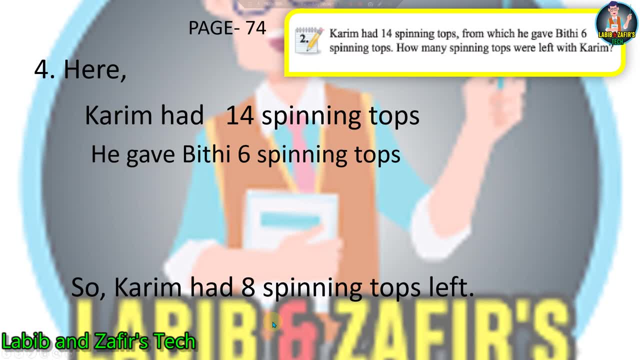 Bithi 6 spinning tops, So here. so Khorin had 8 spinning tops left. because if we do here, the calculation we get left: 14 minus 6 is equal to 8 spinning tops. So that's why Khorin had 8 spinning tops left. So, student, this is our today's fourth word problem. 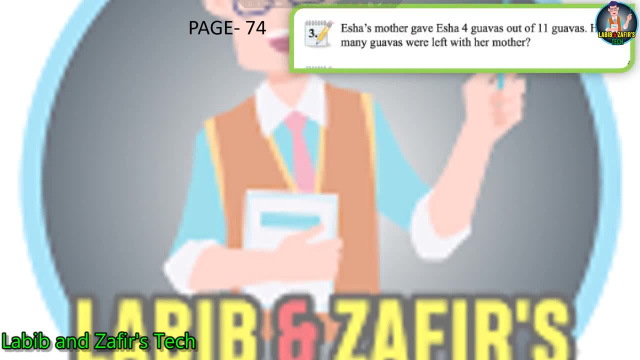 Now let's go to our fifth word problem. So here is our fifth word problem and the question is: Isha's mother gave Isha 4 gobas out of 11 gobas. How many gobas were left with her mother? So we can see in the question that her mother had 11 gobas and the mother gave. 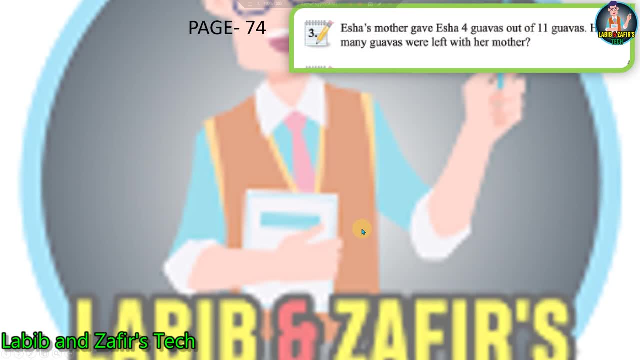 11 gobas. So we can see that her mother had 11 gobas and the mother gave 11 gobas. So we can see Isha 4 gobas. So we have to find the number of gobas left with her mother. So number 5,. 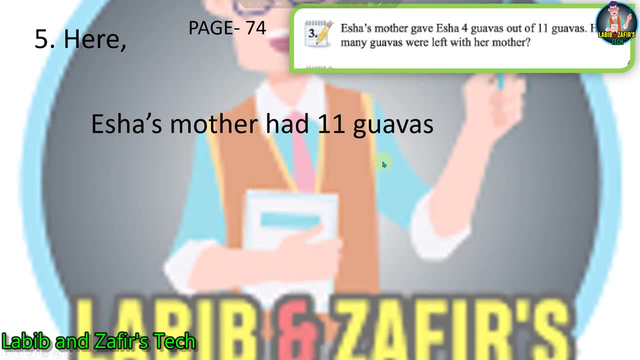 here. Isha's mother had 11 gobas. Isha got 4 gobas. So if we do the subtraction here, then we get 7 gobas, because if we add 7 plus 4 is equal to 11.. So after 4, if we calculate, 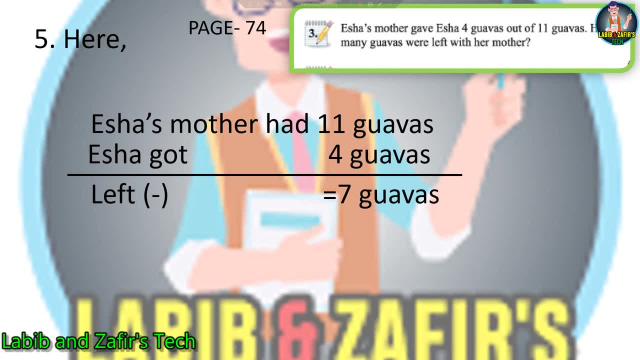 5,, 6,, 7,, 8,, 9,, 10,, 11.. So at the 7th position, or 7, we get the 11 number. That's why 7 gobas. So 7 gobas were left with Isha's mother. 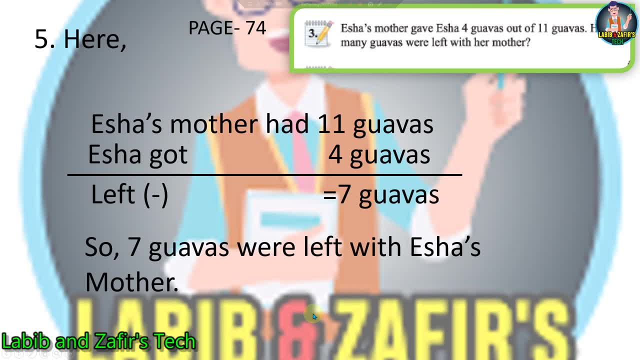 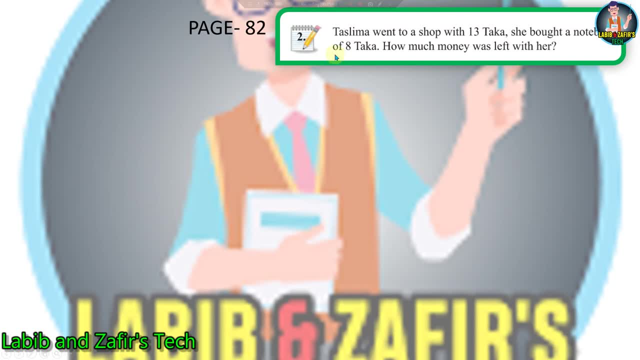 So, students, this is our fifth word problem. Now let's go to our next word problem. So this is our next word problem. From page 82,. Taslima went to a shop with 30 thaka. She bought a notebook of 8 thaka. How much money was left with her? So, students, we can see this. 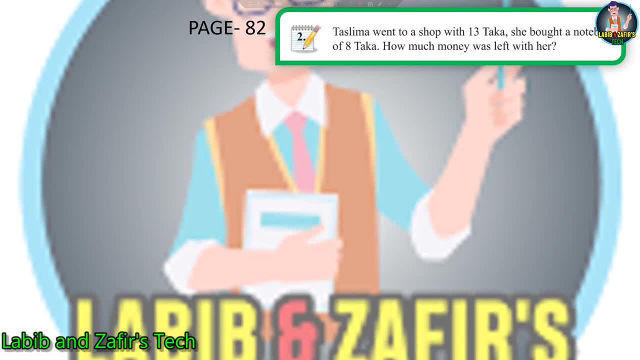 is a new type of word problem. So we can see that she bought a notebook of 8 thaka. How much money was left with her Related with money? So let's see the solution. So number 6, here Taslima, had 13 thaka. She bought for 8 thaka. Then if we do the subtraction, then 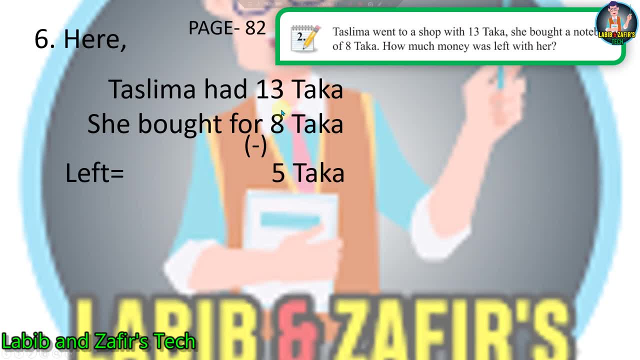 we get 5 thaka, because Taslima had 13.. And if we subtract 8 from 13, we get 5.. So to prove it, we, If we add, If We could, If we add 8 plus 5, then we get 13.. So 5 tagger was left with Taslima. So, students, this is our 6th word problem. Now let's go to our next word problem. That means 7.. 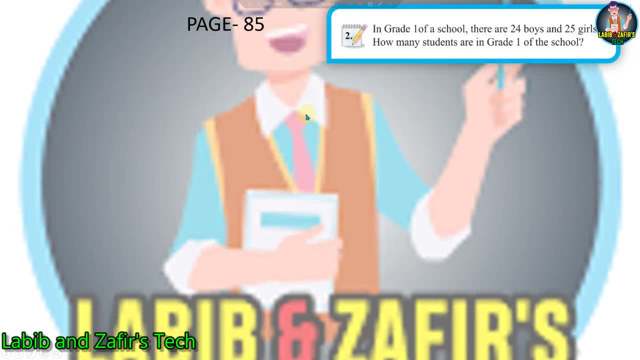 So, students, now we are in page 85 and this is the question here. In grade 1 of a school there are 24 boys and 25 girls. How many students are in grade 1 of the school? So, students, we can see here that there are 24 boys and 25 girls in a grade 1 or class 1 school and we have to calculate the number of students in that class of the school. 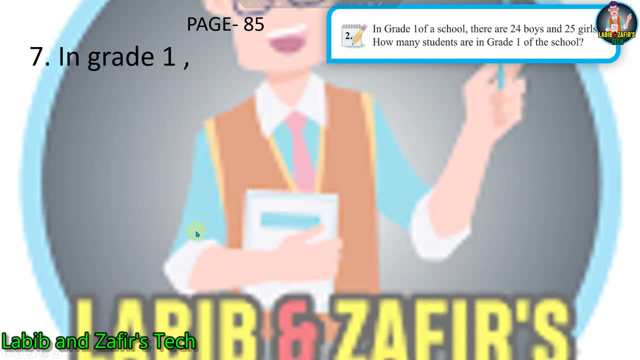 So how many students are in grade 1 of the school? Here is the solution: In grade 1 there are 24 boys. There are 25 girls. So if we do the addition here, then we will get 5 plus 4 is equal to 9 and 2 plus 2 is equal to 4.. That is 49.. 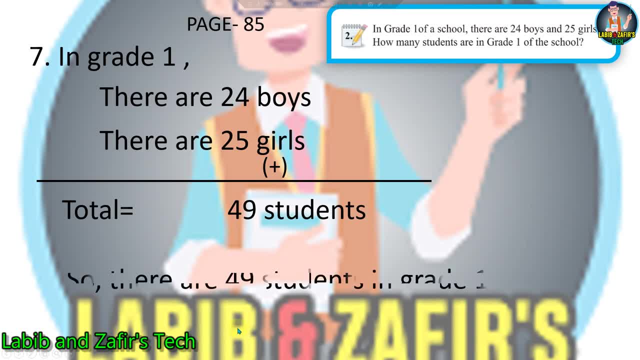 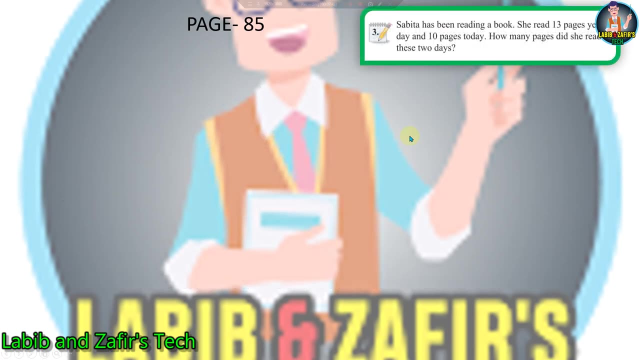 So total 49 students. So there are 49 students in grade 1.. So, students, this is our 7th word problem. Now we will go to our next episode And the last word problem of today's video. So, students, this is our today's last word problem from page 85.. And we can see the question. 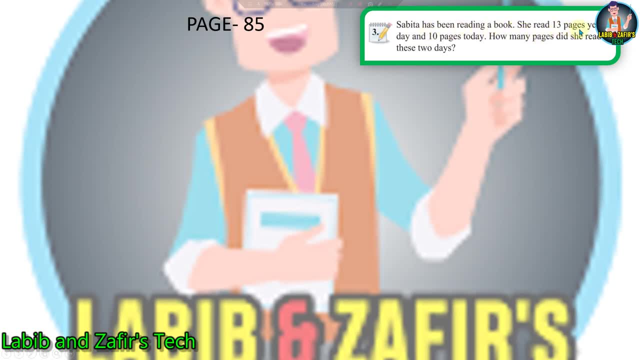 Sabita has been reading a book. She read 13 pages yesterday and 10 pages today. How many pages did she read in these 2 days? So, students, we have to find the number of pages she read in total in these 2 days. So we have to add these 13 and 10.. Then we will get the answer. 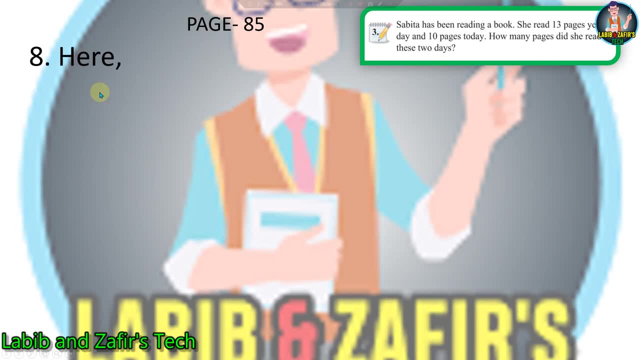 So 16.. So this is the solution Number 8 here. Yesterday she read 13 pages, Today she read 10 pages. Then we have to add this thing. Then if we add, we will get 3 plus 0 is equal to 3 and 1 plus 1 is equal to 2.. That is 23 pages. So total: 23 pages.